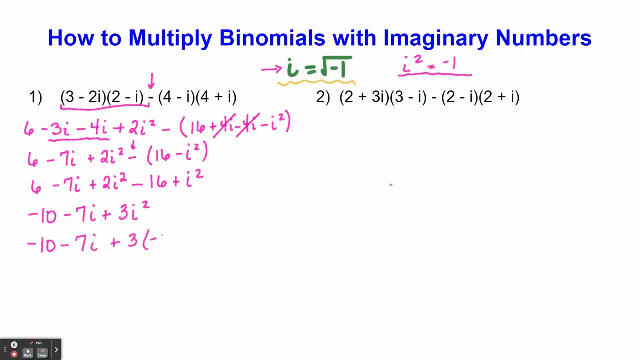 So I'm going to replace this i to the second with a negative one, And of course, three times negative one is going to give me negative three And I can combine like terms with the negative 10 then, So that I get negative 13 minus. 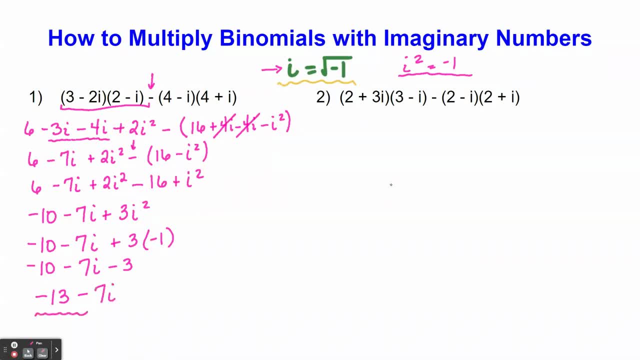 seven i, And this is my final answer there. Now I want to do one more, because I always find that the second example helps us to kind of solidify the process. So let's start here on problem number two, the same way we did on problem number one, by distributing or using the full method with 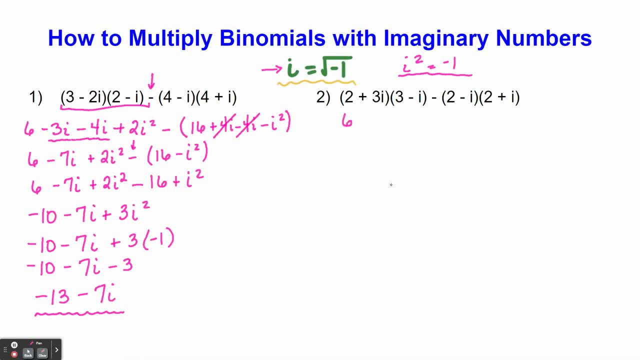 these first two parentheses. So two times three would give me six. Two times negative, i would give me negative two i, Three i. or times three would give me nine i. And then three i times negative, i would be negative three i to the second. Again, I'm going to hold that minus out till after I do the multiplication. 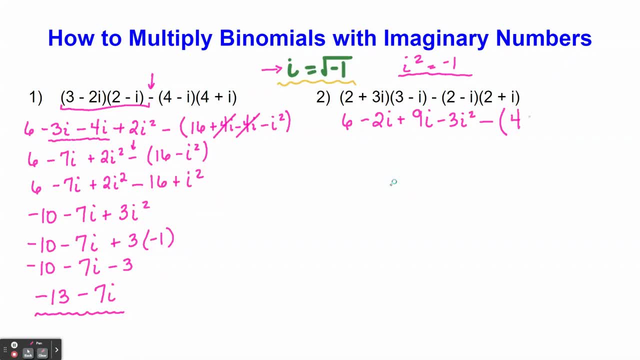 So two times two is four. Two times i gives me two i. Negative i times two gives me negative two i. And then negative i times i gives me negative i to the second. All right, I'm going to combine like terms out here. 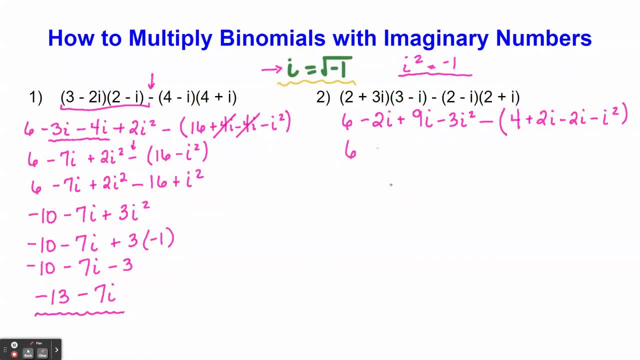 So I've got six and then minus two i plus nine, i gives me seven i, And then I'll just go ahead and cancel those two. i's inside that parentheses And now I'm ready to distribute that minus. that's out in front of the parentheses here. 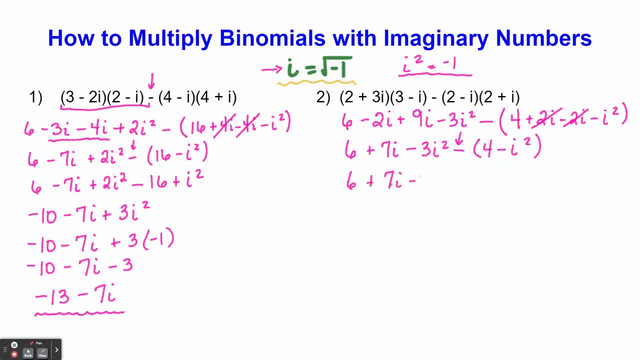 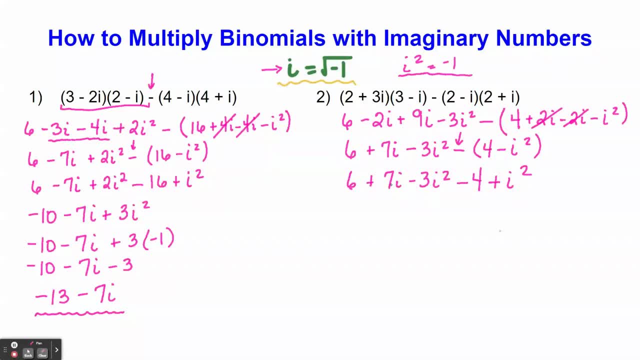 me positive. i to the second. All right, Just like before, we'll combine like terms: The six and the negative four give me two, And then the minus three out of the second plus i to the second gives me negative two. i to the second. Last step: we'll go ahead and make the substitution that i to 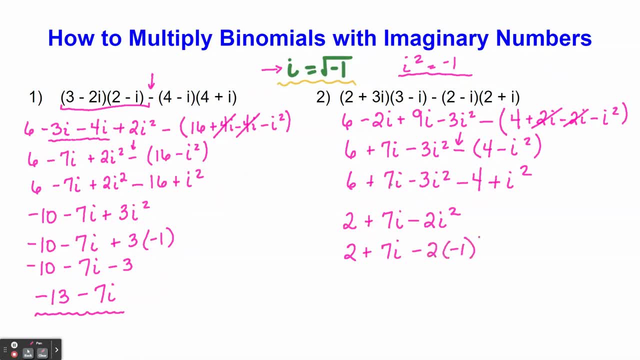 the second is negative one, And so that gives me minus two times. negative one is negative two. So now I can change that to adding a positive And we can combine like terms. Then again four plus seven, i, And again you see my final answer there. I hope this helps. you see the pattern between the two. 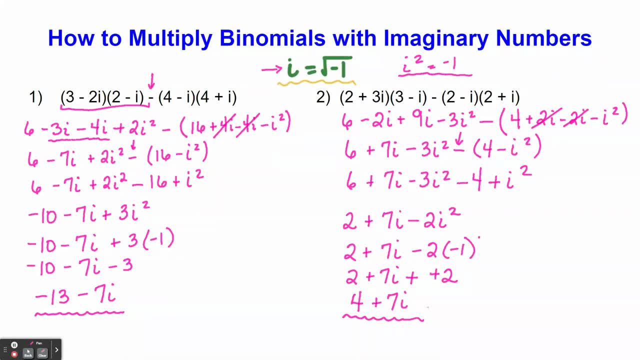 That we did the same process. Take your time. There's a lot of sign, you know, changing of positives and negatives. So I'm going to go ahead and do that, And then I'm going to go ahead, and I find that students often make a mistake with that. So be very detailed in your work, as you're. 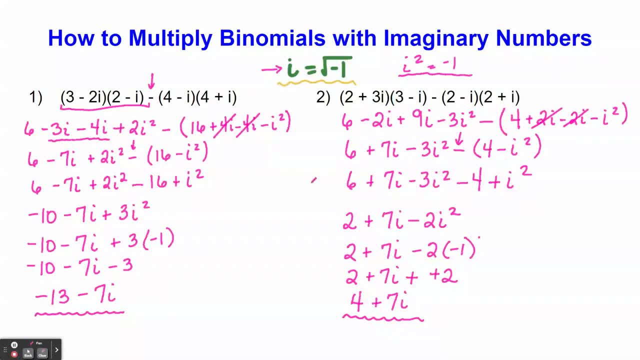 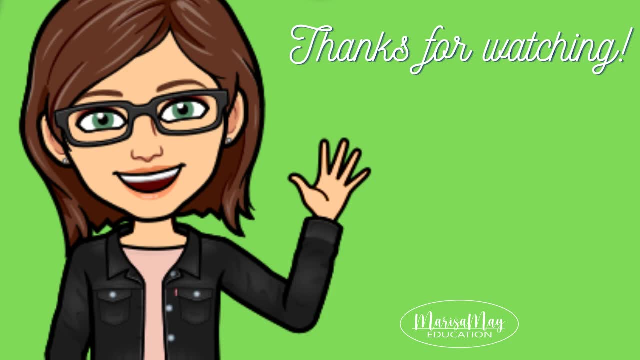 working these type of problems And I think you'll avoid those mistakes. All right, Bye for now. Bye for now.